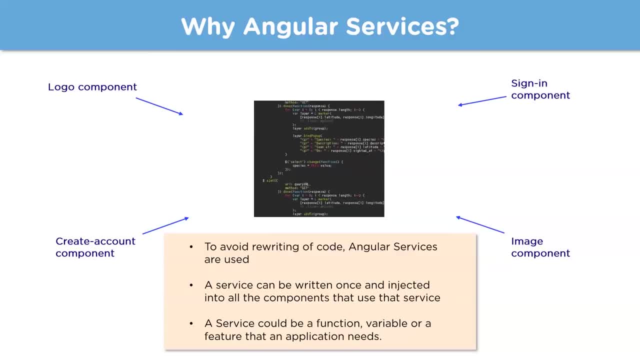 a variable or a feature that an application needs. So the main use of a service is to write code once and avoid rewriting of it. Now the same code can be injected into several components that make use of this particular service. But what are Angular services Normally? 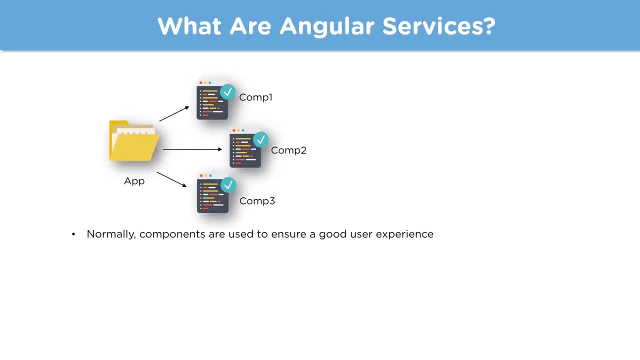 to ensure a good user experience. Now, that is the extent of it. Components make sure that whatever is being rendered onto the screen is right and pristine, But in order to execute tasks, we make use of services, and this approach is ideal. So a component can basically delegate. 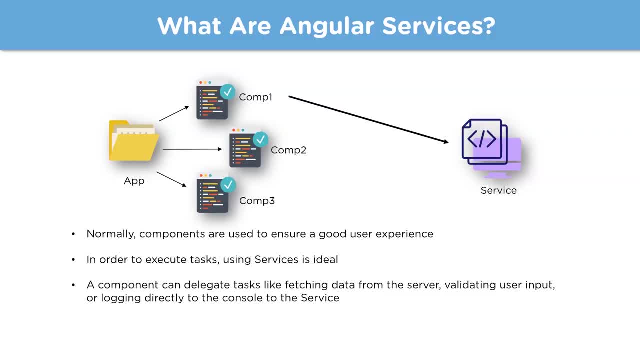 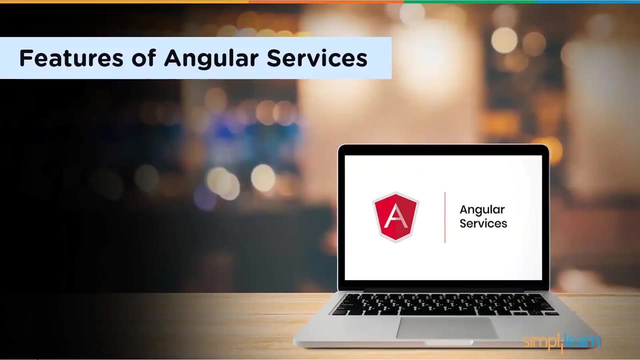 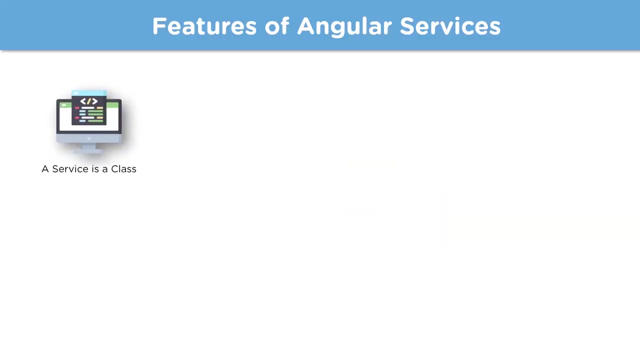 tasks like fetching data from the server, validating user input or logging directly to the console to a particular service, And these tasks can be made available to any component in the app. So now let's talk about a few features of Angular services. Now. typically, an Angular service is simply a TypeScript class with an at injectable decorator. 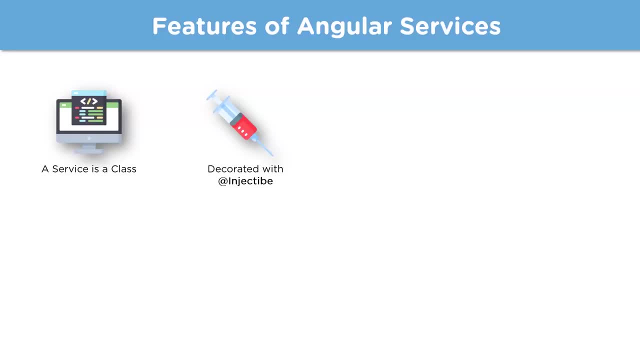 This decorator tells Angular that the class is a service and can be injected into components that need that service. Now they can be used to share the same piece of code. They can also inject other services as dependencies. Now these services hold valuable business logic and can also be used to interact with the backend. Now, for example, if you want, 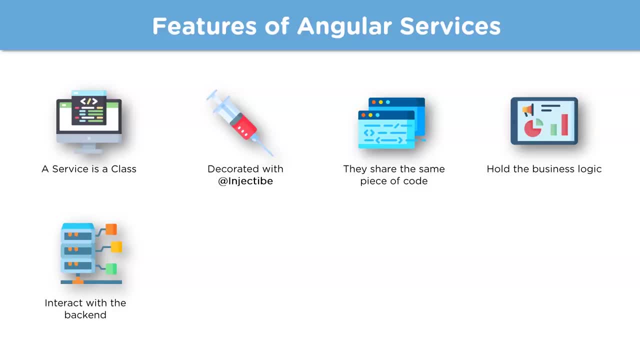 to make Ajax calls. you can have methods to those calls in the service and then use it as a dependency in files And, as mentioned earlier, it can be used to share data among several components. In Angular, services are singleton, meaning that only a single instance of a service gets. 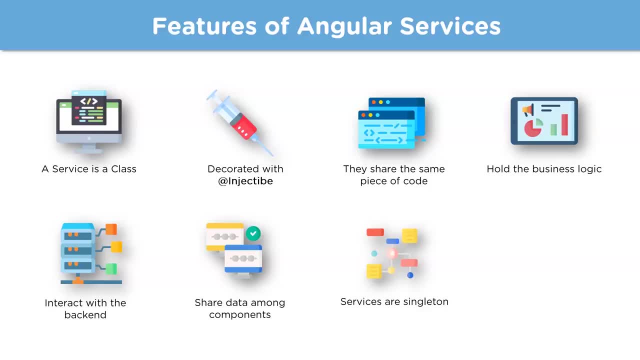 created and the same instance is used by each and every building block in the application. And finally, a service can be registered as a part of a module or it can be registered as a part of the component. Now, to register it as a part of the component, you'll have to specify it in the providers. 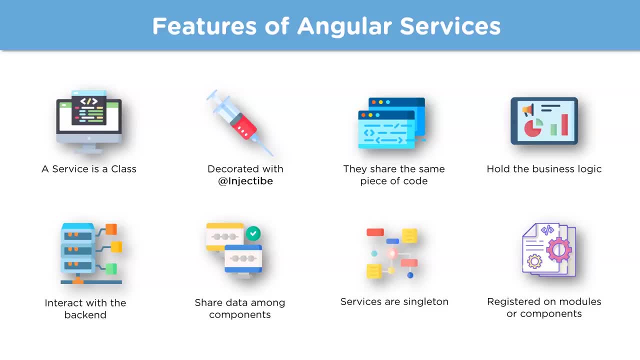 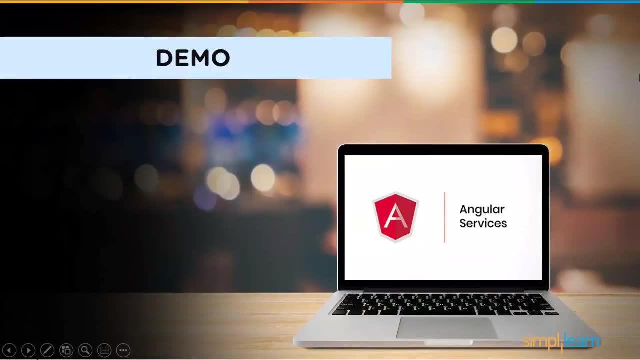 array of the module. I'm sure you'll understand the concept of services better if we look at a simple demo. So in the next section we're going to look at a demo, But before that let me tell you the use case. 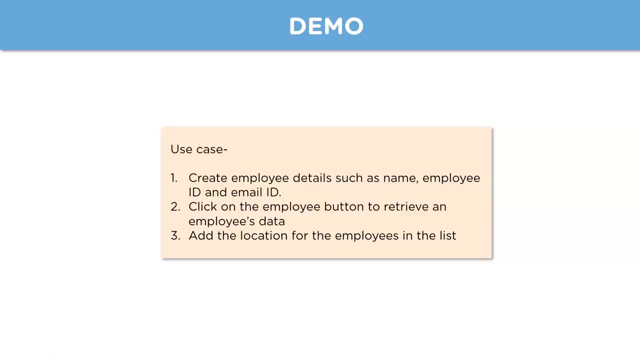 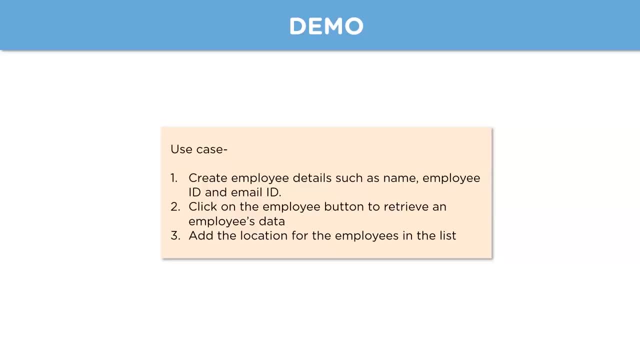 the browser. when you click on the employee button, it displays the information about that particular employee, And at the end we can also add information to the employee's details. So without delay, let's head to our VS Code and start learning Angular services hands-on. So here first, 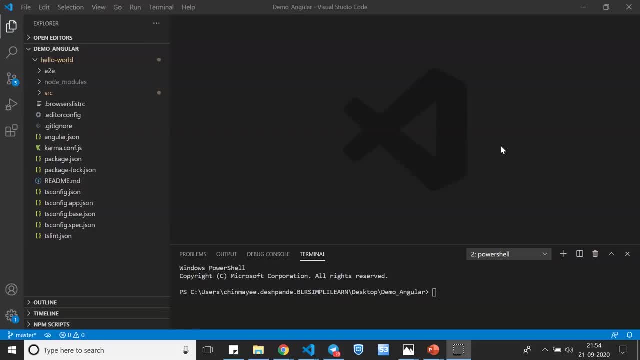 I've created a folder called demo- underscore- Angular, Within which I've created a file called hello world. So this was previously used for a tutorial, So the name is just hello world, So don't get confused. However, when you look at the 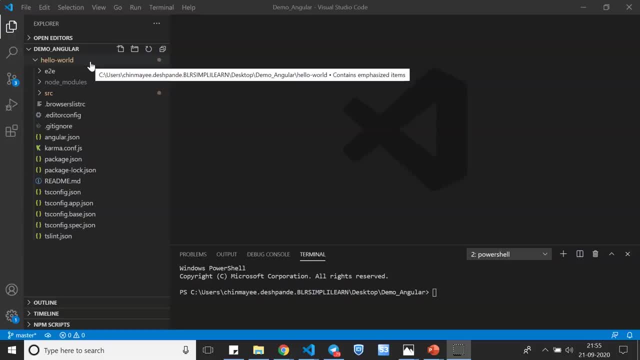 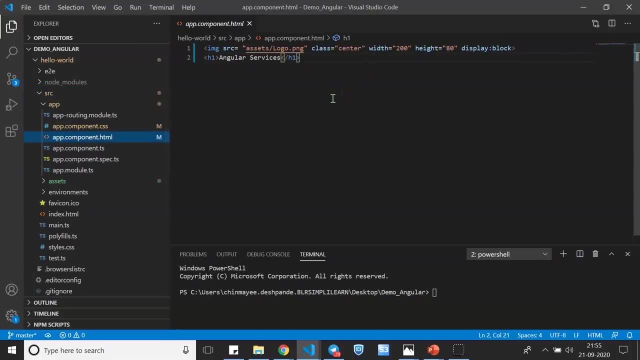 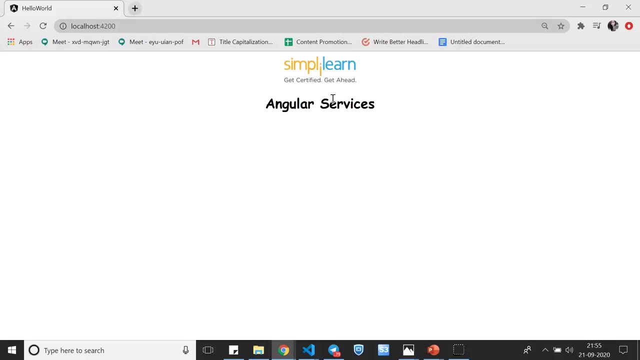 browser. I've written an initial code here which is Angular services, And I have the Simply Learn logo. So back in my browser, this is what the UI looks like, So to. So to understand the concept of Angular services, first let's go ahead and create a component. 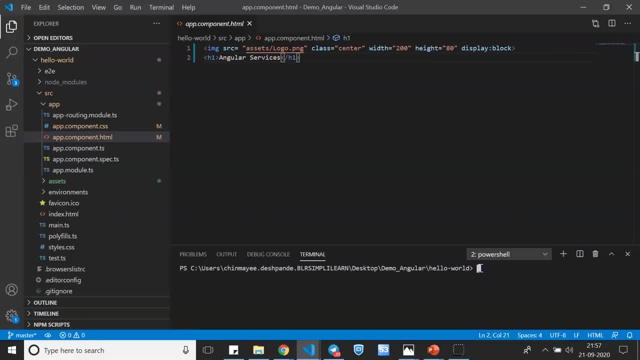 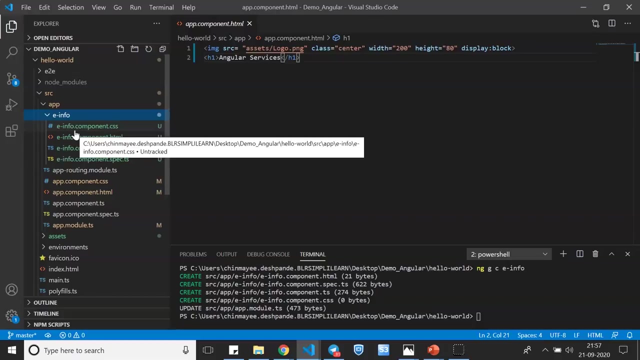 So here I'm going to say ng gc, e-info. I'm creating a component for employee information. So, as you can see, inside my app file we have the e-info component which has these four files. So if you're wondering what exactly components are and how this is working, then I highly 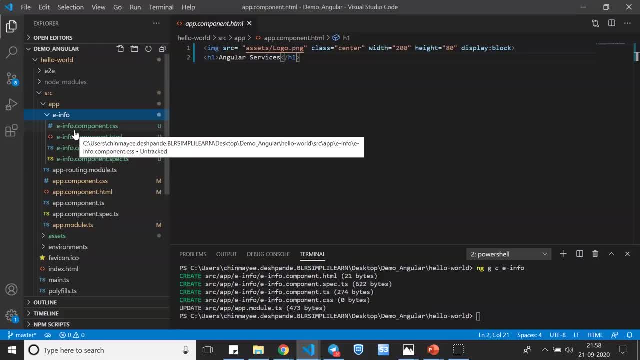 suggest you watch our components video first. So now let's go ahead and create a service. So I'm just typing in the command ng gservice. Here g stands for generate And we're generating a service, and the name of the service that I'm providing is data. 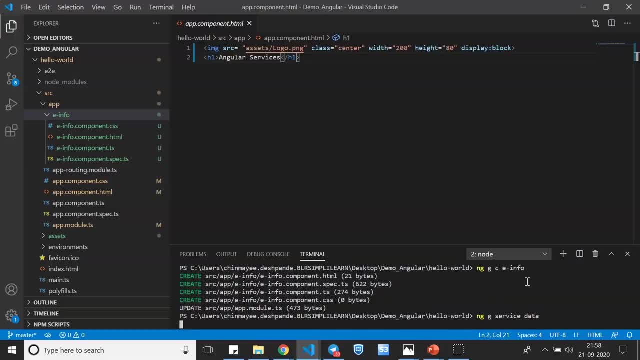 So now it creates a service. It's going to be a ts file, So you can observe that service is appended. This indicates that it is a service. all right, As mentioned earlier, we have to display the employee details, correct. 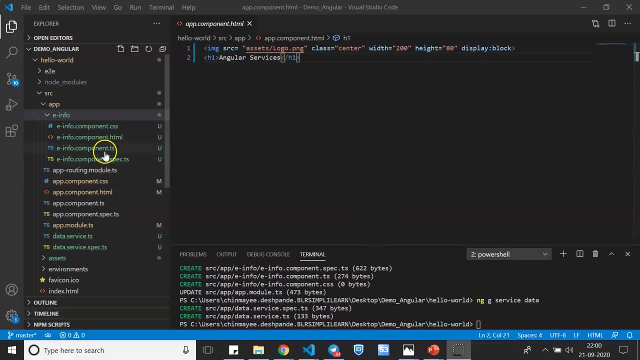 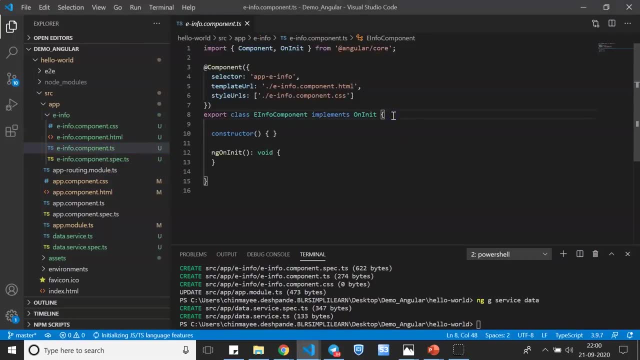 So for that, in my componentts file, I'm going to create an array that displays the employee information. In our case I'm creating three different employee records, So for that I'll have three different arrays. So let me just call the arrays info receipt, one indicating this is the information of 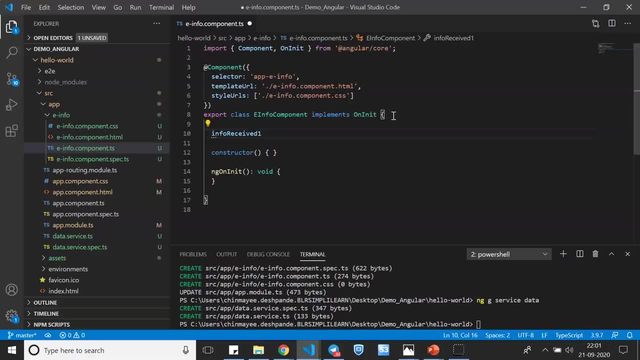 first employee, And this is going to be of type string And I'll just initialize it to null for now. all right, And I'm going to create two other arrays And that's it, All right, And let me just change the name of the arrays. 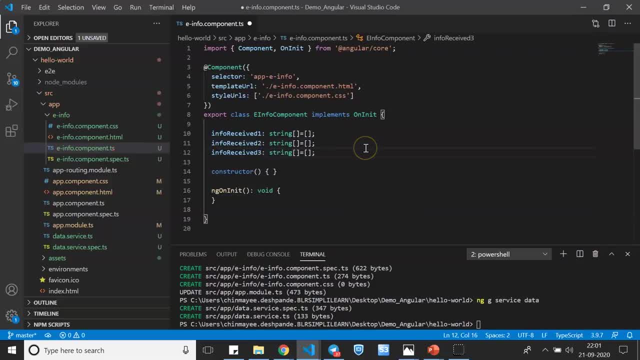 All right. So now to retrieve the information, I'll have to create a method Again. I'm creating three methods for the three different employee records. So I'm going to call the array getInfoFromService one, indicating it's again for employee. 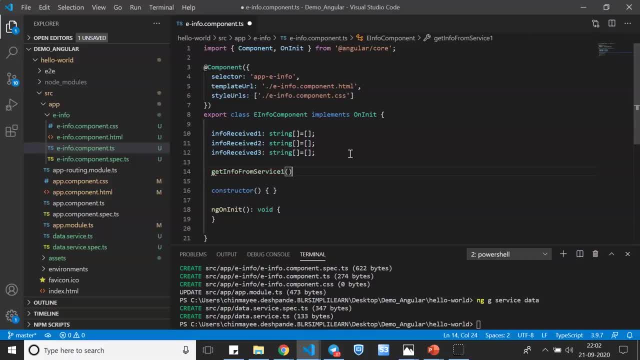 one, And I'm just going to leave it as it is for now. I'll tell you how the information is being received, And I'm going to do the same for the other two employee records, So let me just copy-paste. 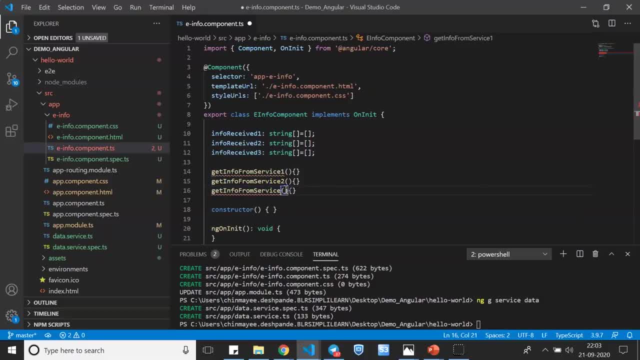 And here I'm just going to change the name of the methods. all right, So this is the initial code for retrieving information. However, we'll have to create the employee record in our server, All right, So I'm just going to call it getInfoFromService. 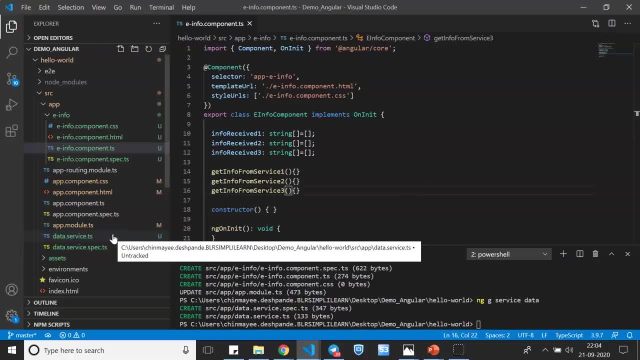 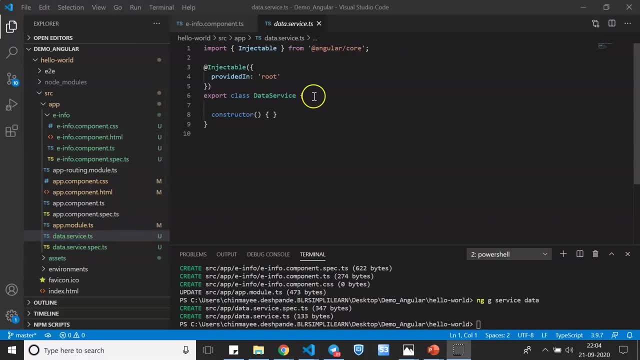 So, back here in my datats file, what I'm going to do is I'll create three different records for the employees. So let me say info1,, which is going to be of type string, all right, And let me just give random names. 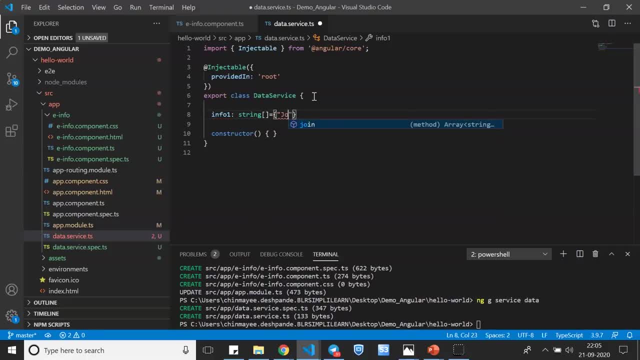 Say, for example, datats: All right. For example, I say John Matthew, all right. And employee ID say E354.. And let me just give a random email ID and say jm at abcnet, All right. So I'm going to do the same for the other two records. 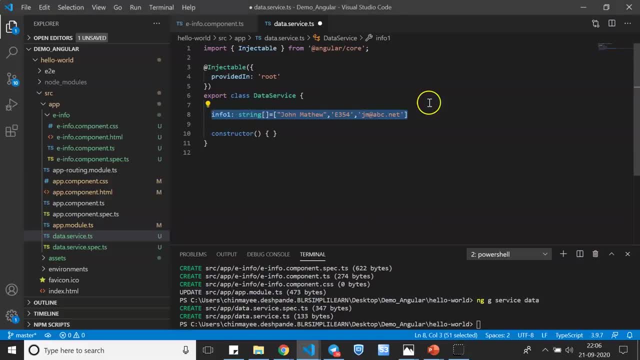 All right, All right, so let me just create another one and call it info2, and the name I'm providing is, say, Rob Wilson, with a different employee ID, say 673, and I'm just going to make it rw at abcnet. and another record. 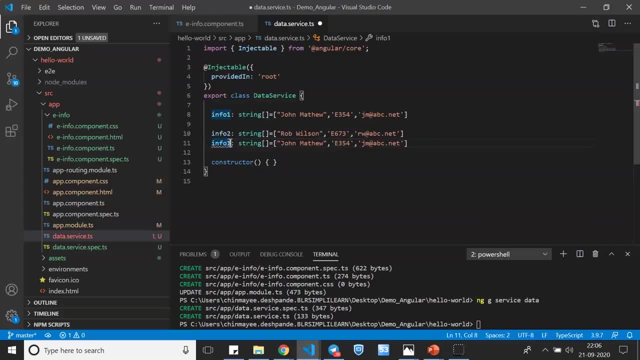 for employee number three, and I'm just gonna say rose Adams, with some employee ID and an email ID. alright, so now we've created the employee records. so what I have to do is I have to create an, a method that returns these employee records. correct, so for that I'm just gonna create another. 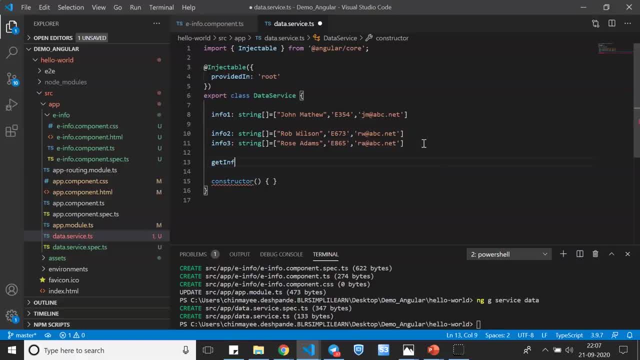 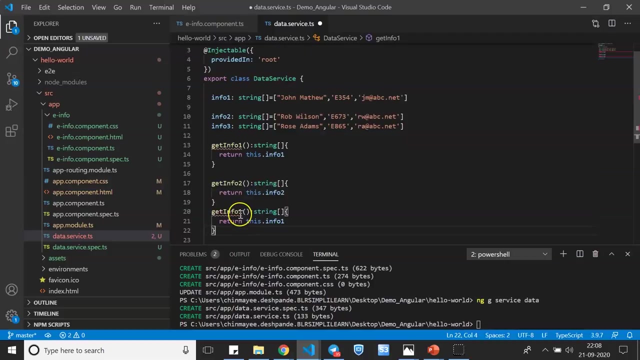 method called get info one, which is of type string, and it just returns this dot info one. all right. similarly, for the rest of the two records, I'm just going to retrieve them and let's say info two and get info two, and again I'm just gonna make it get info three and this: 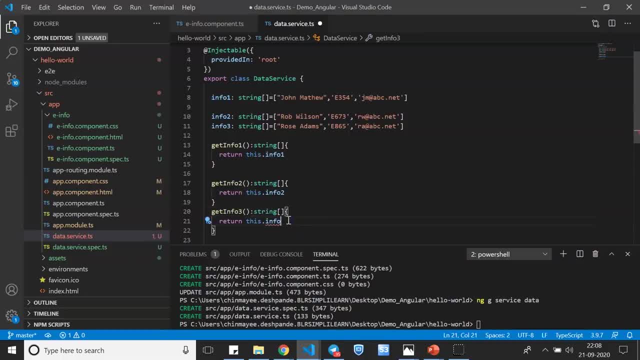 is gonna return info three. all right, so I'm sure you've got an idea as to what I'm doing here. so basically, this information is going to be retrieved in our employee component, correct? so for that I'll have to make use of dependency injection. so here I'll have to import the service. 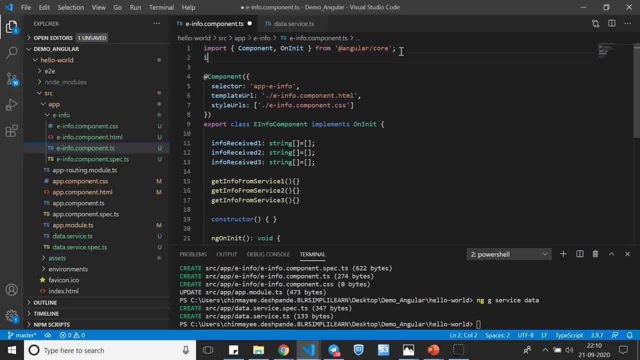 that I've created. so let's go ahead and say: import the service with data service- all right, from slash data dot service- all right. now, the main reason we are doing this is to tell angular that when the component is created, the service instance is also created, and this instance is being used to perform particular tasks and for 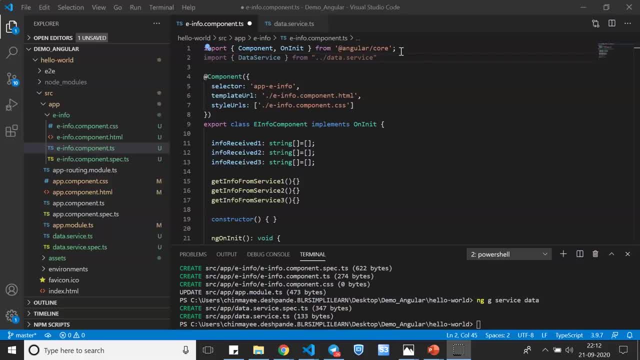 that we also have to include this in our providers array. so here let me just say providers and let's say data service. now, to access this instance of service that is created, we make use of a property. so, uh, this property basically allows us to access all the methods that are defined in the service class. 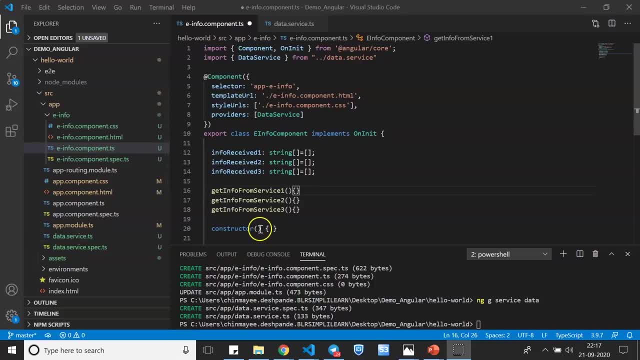 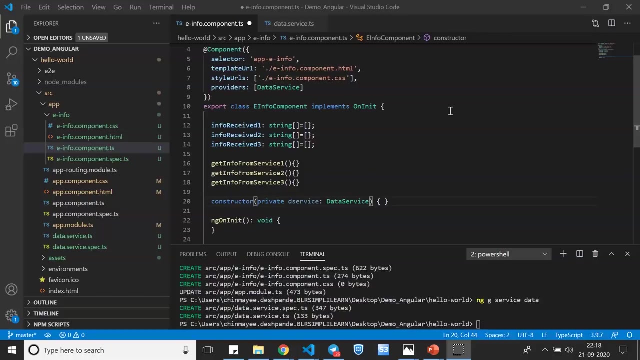 all right. so here, in my constructor method, I'm just going to say private and you can give any name for your property, and here I'm just giving the name D, service, and which is of type data service. all right, so now, with the help of this property, I can retrieve information from the service class. 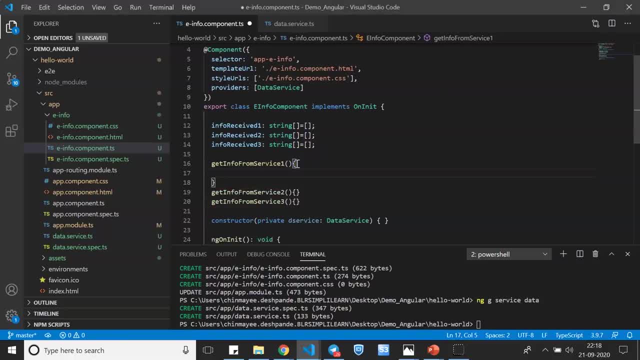 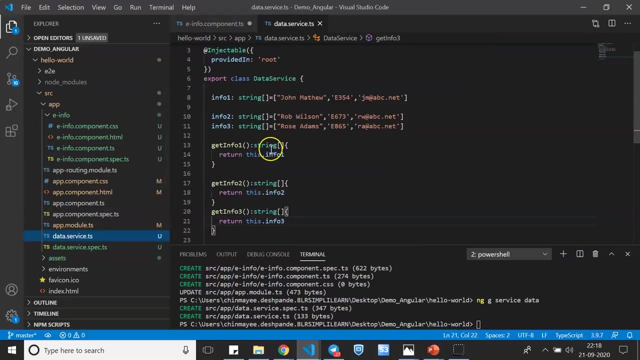 so here I'm just going to say this: dot info receipt equals this: dot D service, dot get info one. all right, so what it basically does is that it calls the get info one, method in our service which returns the information of the first employee, and this information is being 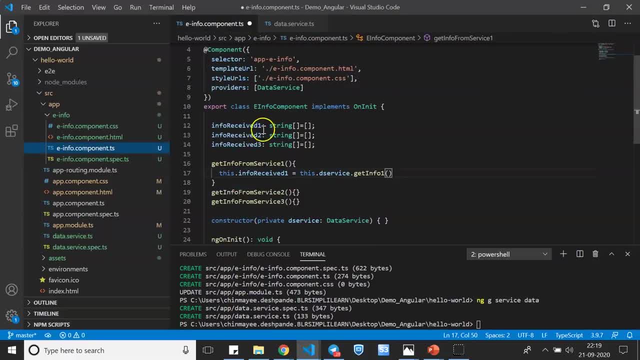 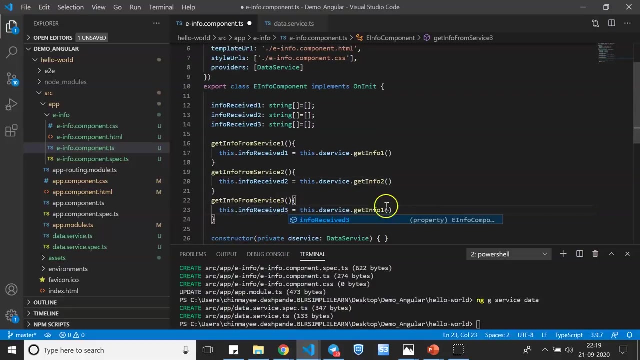 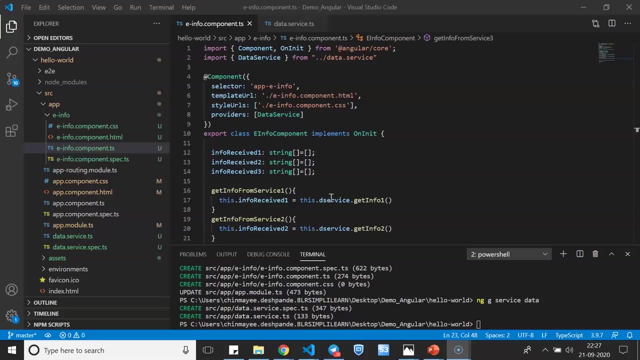 stored in the array, that is, info received one. so similarly for the next two methods, I'm just going to use the same piece of code and just change it here, and same for the third one, all right. so now that we have the logic behind what is being displayed, let's go ahead and create. 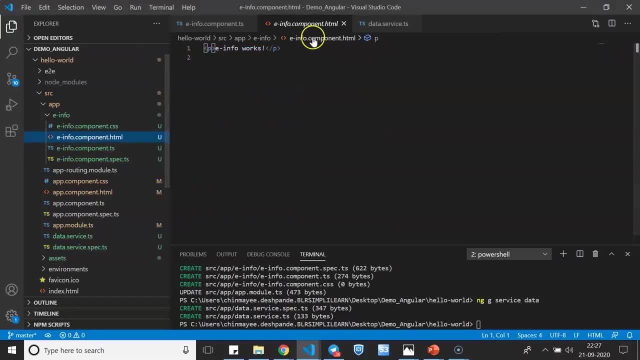 the UI for it here in my HTML file I'm going to create an unordered list and now I'm going to make use of the ng4 director to uh, basically loop over the record and display everything. so for that I have to make use of a particular variable. so I'll just say: let info off, info received. so, um, you can checkó. 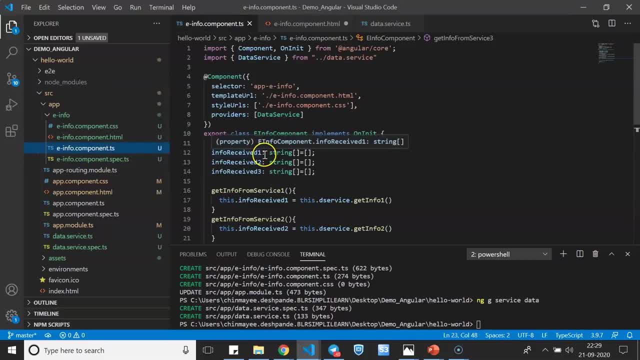 frontline button now, which is the command of the UI for this one table. um, I'm going to click over here in this one frame. I'm then going to enter information here, which means I'm going to assign input for info receipt in our ts file. the array is info received, correct. so i'm going to make use of the same array here. 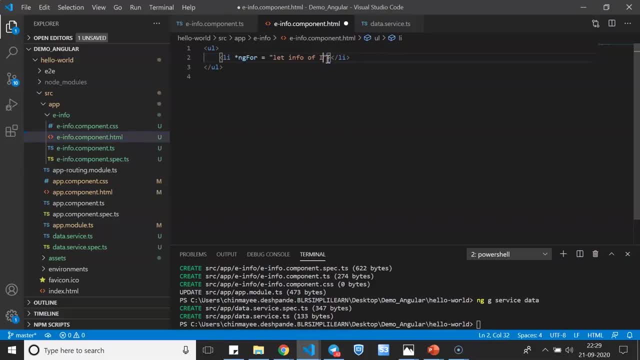 and since it's displaying the first employee record, i'm just going to say: info received one. all right, and let me just create a class, a bootstrap class, of list group item of list group info, and we're just gonna have to interpolate info. all right, that is basically going to display what the information holds, what the info variable holds, all right, and 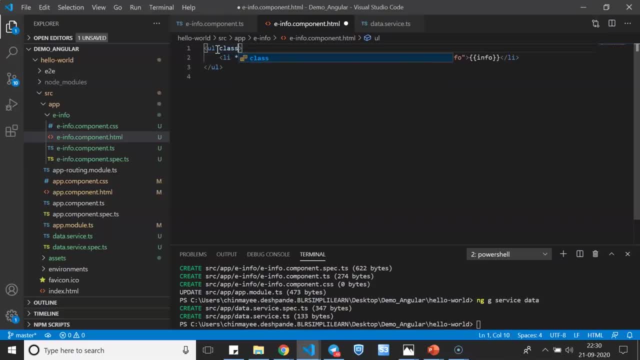 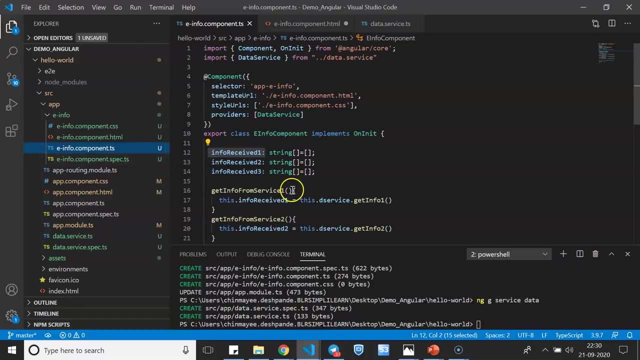 here as well. let me create a bootstrap class called list group, all right? all right, i hope this was clear to you. so, basically, here the information is being retrieved with the help of this method, right, that is, get info from service one. so in order to call this method, we'll have to bind it with a button. all right, so that's. 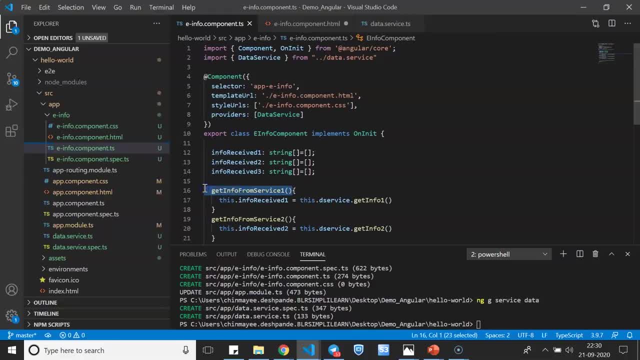 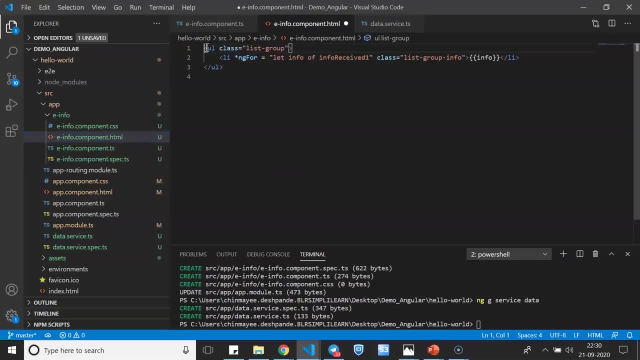 what we're going to do. let's just copy this, and here i'm going to create a button, all right, and the type is: button with name button, again all right. so i'm going to bind it with the click event. so what happens is that when i click on it, this particular method gets called. all right, i'm just facing the method. 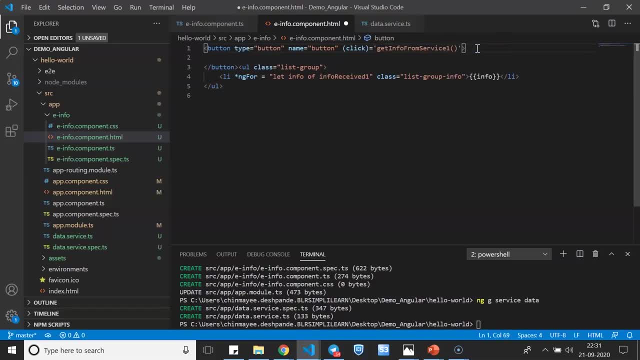 here. and finally, let's just provide the name employee one for the button, all right? so, uh, similarly, we'll have to do the same for the other two records as well. let me just make this look better, all right. so, uh, what i'm gonna do is i'm just gonna paste the same twice, and here: 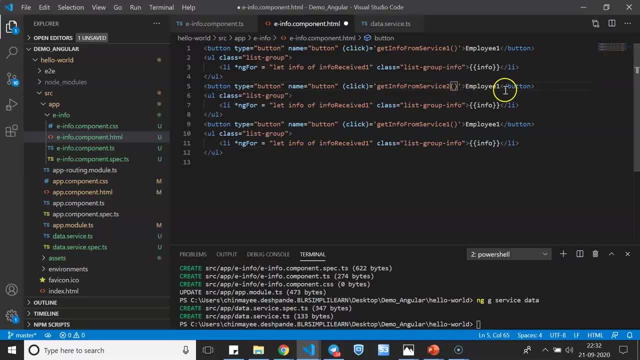 i'm gonna just change the names. i'll say two here and this is again for employee two, and i'm going to change this as well. it's going to be employee. i'm sorry, it's going to be info. received. two: this is going to be in four: received. 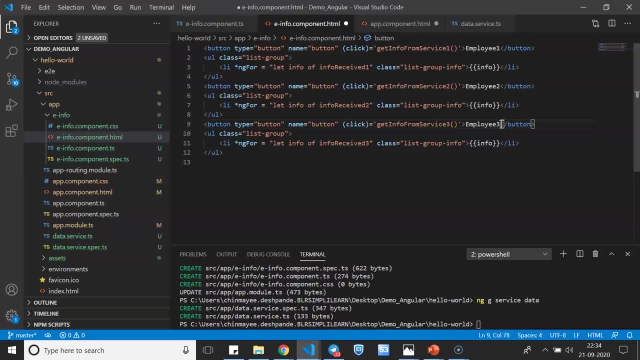 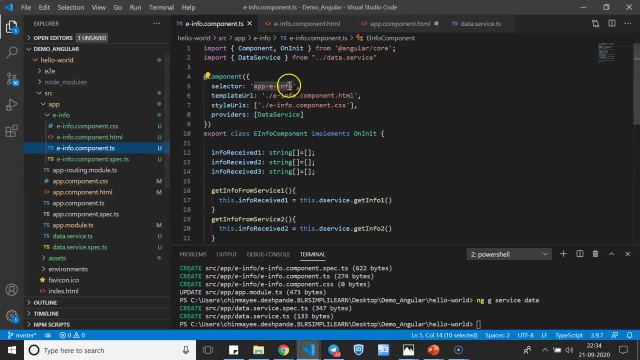 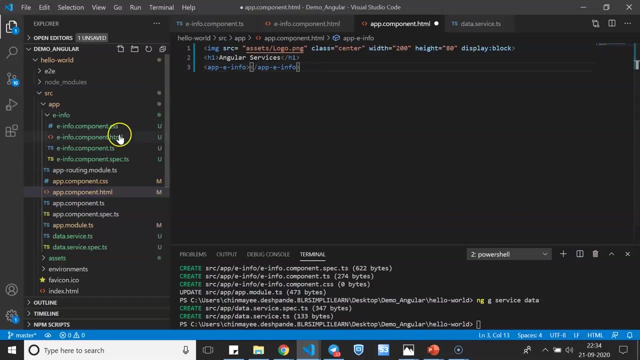 three, and finally, employee three. all right, uh. and lastly, we'll have to include the selector, that is, app hyphen e-info, in our main component or HTML. so here let me just create a custom tag, all right, and save this. so now let's go back to our browser and see what it looks like. 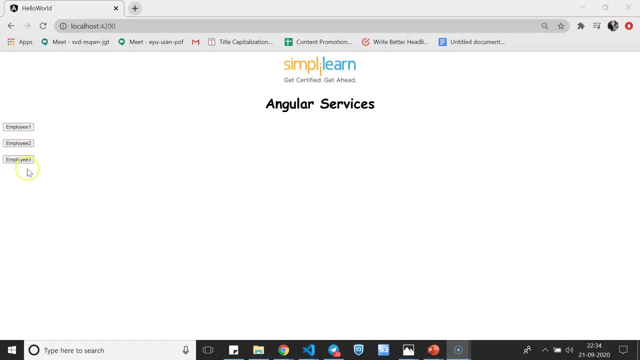 so here you can see that three different buttons have been created for employee one, two and three, and when you click on it it retrieves information, that is, the name, the employee ID and their email IDs. so we've successfully created an angular service and injected it into our component to retrieve information all. 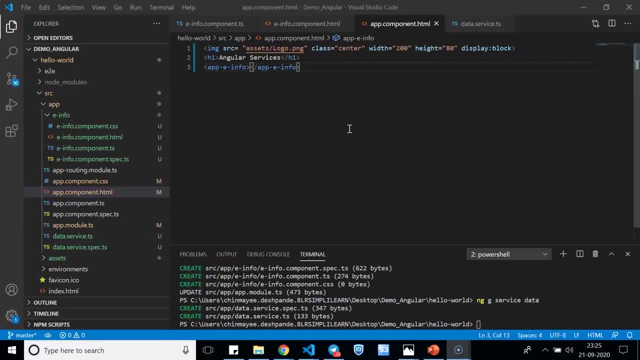 right, so now, the last part of the use case that we discussed was to add another detail, that is, the employee detail in the record. all right, so for that we'll have to take input from the user and in our case we're taking the location. now, we're all. 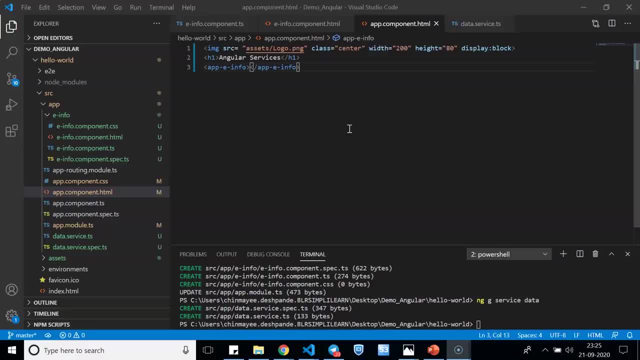 adding the same location for all three employees. so this is what services do you know? they can be used to update, modify, alter anything that happens in the backend, so you can tweak the code a little bit and you can change the entire view of your application. you can add information, you can, delete. you can. 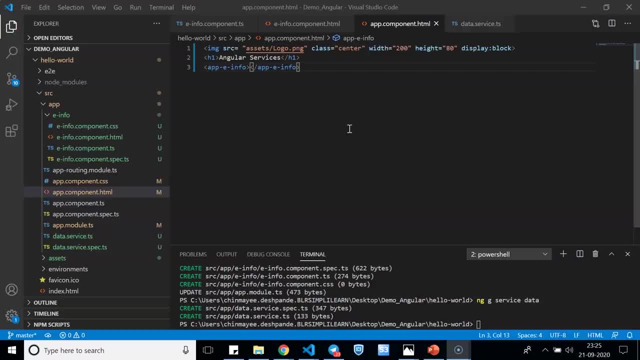 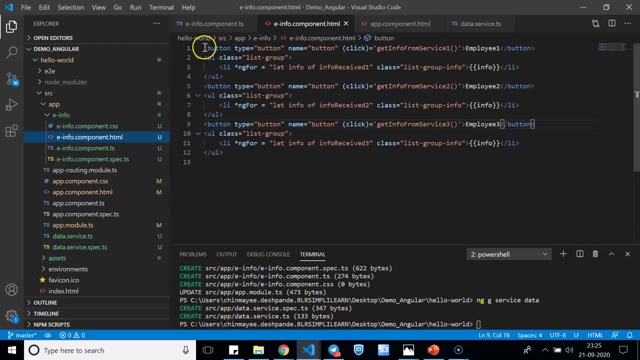 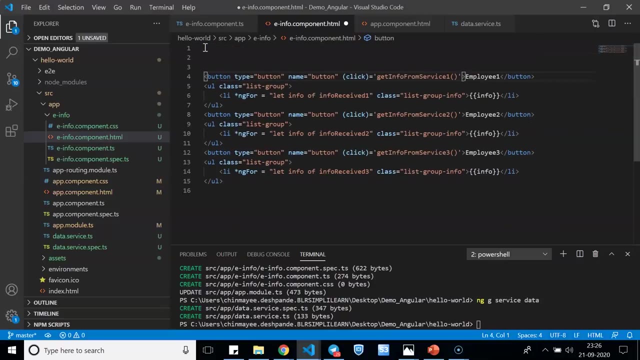 retrieve, you can alter, etc. all right. so for that, what we're going to do is, back in the HTML file, we'll create a form that basically takes the input. so I'm just going to say form, all right, within which I'm going to be defining a div. 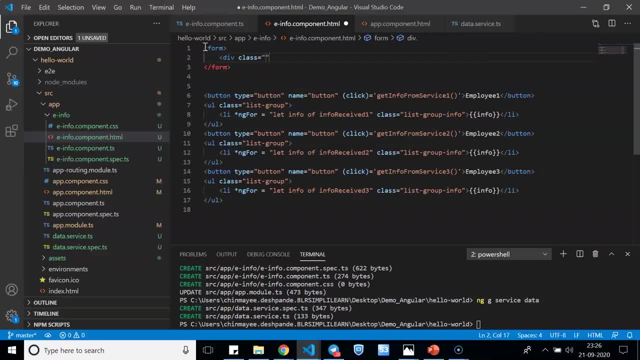 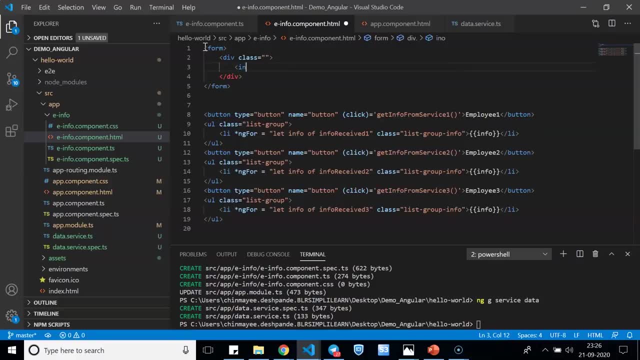 class within which I'm going to be defining a div tag inside of which I'll have a type of text and the name I'm going to be providing. it will be location, all right, and we'll have a value, and I'll just leave it blank and, finally, I'll have 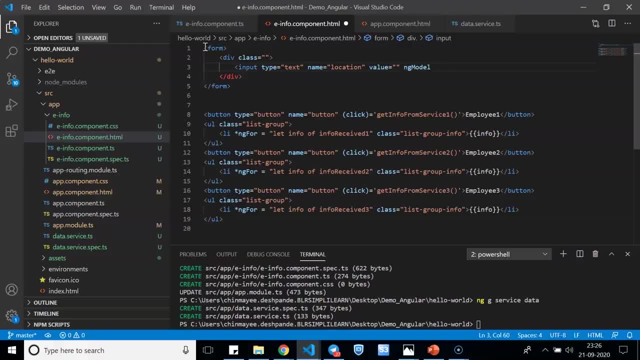 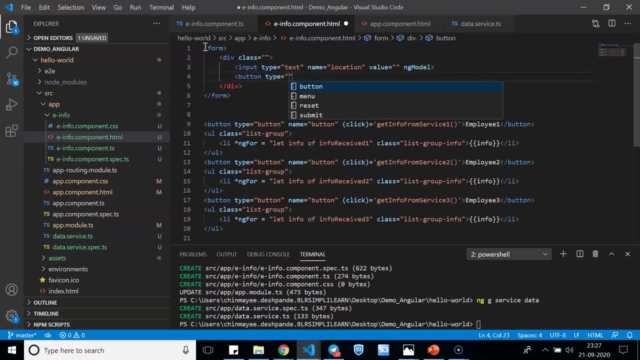 ng model. so if you're confused as to what I'm doing here, then I suggest you watch the angular forms video. it basically teaches you how to work around with angular forms. all right, and now, after this, we're gonna have a button. so let me say button, all right, and I'm gonna just say add info. okay, all right. 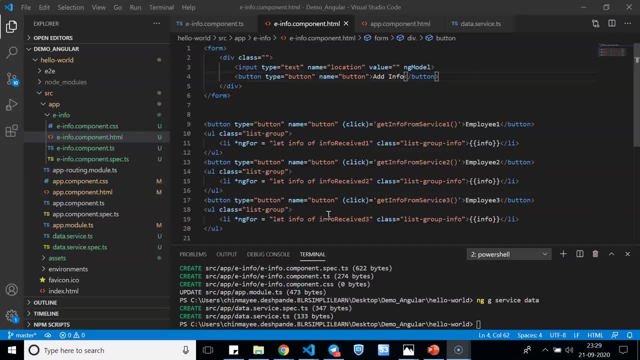 so now, when I'm creating the form, I'll also have to create a template variable to access all the values within my form. so if I have to access the location, then I need a variable to access it. so here let me just go ahead and create a template variable, let me call it frm, and I'm going to make use of 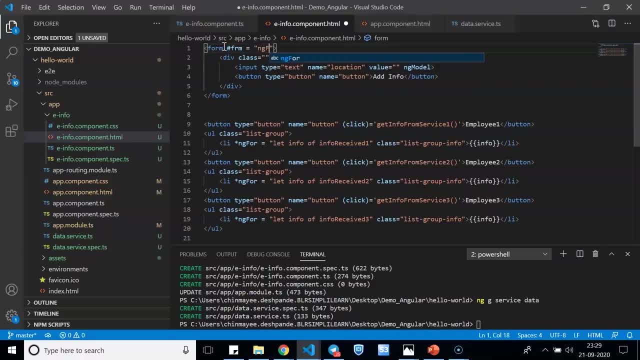 the ng form directive. so this tells angular that this variable can be used to access all the values within the form. so this tells angular that this variable can be used to access all the values within the form. and since I'm using form here, I'll have to import it in my module file. so here I. 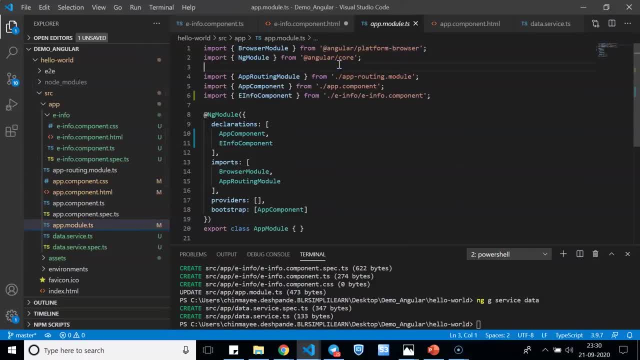 just go ahead and say: import forms module from angular forms and here in my imports I'll just say forms module. okay, so I've imported the forms module, and so now back in my HTML file. what I'm going to do is that I'll have to make 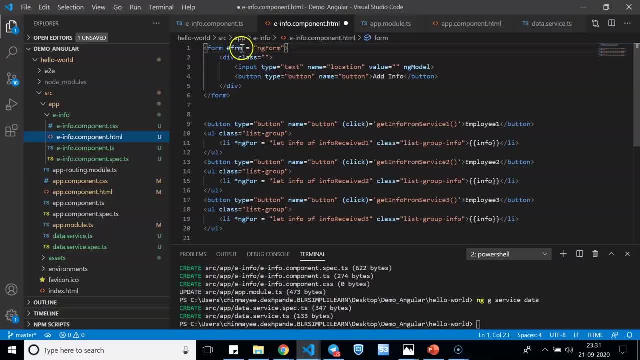 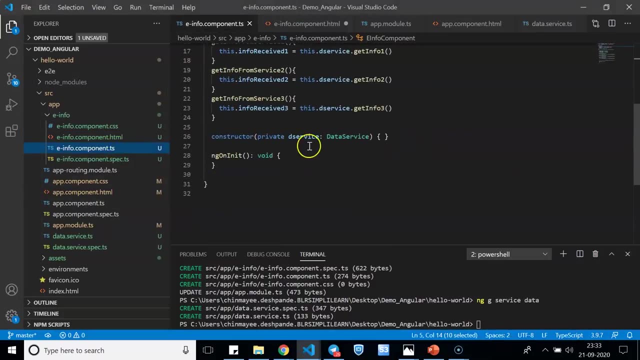 use of this template variable to update my information correct. so I'll have to create another method that will update information into the records. so here in my componentts file I'll have to create another method and I'm going to call this method updatetxt info method. all right, and this basically takes in the template variable, that is. 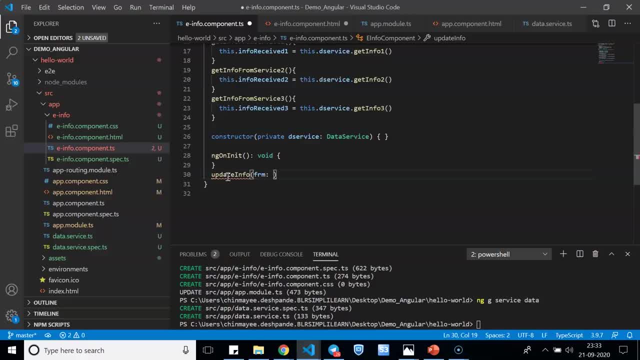 form and let me just specify any. okay, and what this is going to do is that it updates the record, correct? so I'm going to say this: dot D service, dot, add a info. now you must be wondering what add info is. I'll just let you know in a 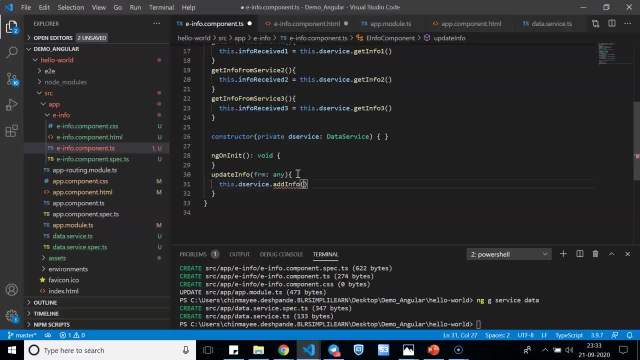 minute, and, and the value that I'm going to be passing will be the value that you've provided as an input, which is nothing but form, dot, value, dot, location. all right, so now what happens is that I'll have to again specify what add info is, and this method is going to be defined in the service file, correct? so? 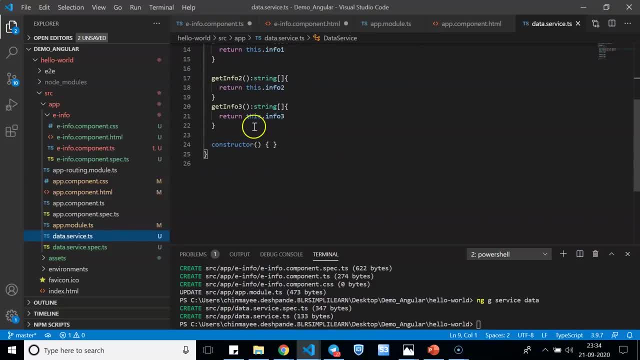 here I'm going to create another method that's add info, and I'm going to pass info as a parameter, and what this method does is that it just pushes the information or the data into the arrays. so since I'm going to be pushing the same information into all of these arrays, that is, info one and info two, so I'm going to 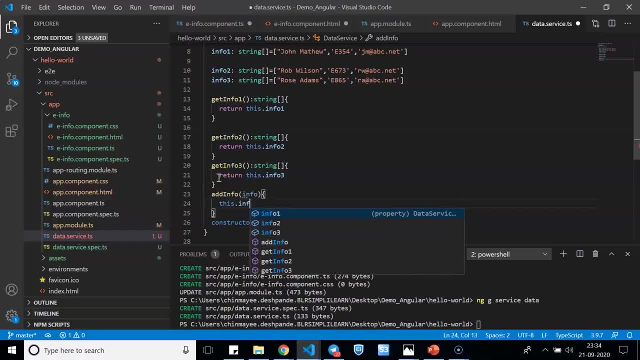 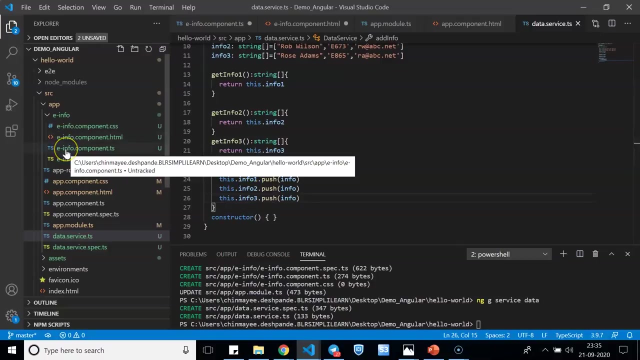 say this: dot info, one, dot push of info, all right, and the same for the other two areas as well. let me just change these, all right. so what exactly I'm doing is that I have I have a method called add info, which gets information and from the component all right, and it basically pushes this information into 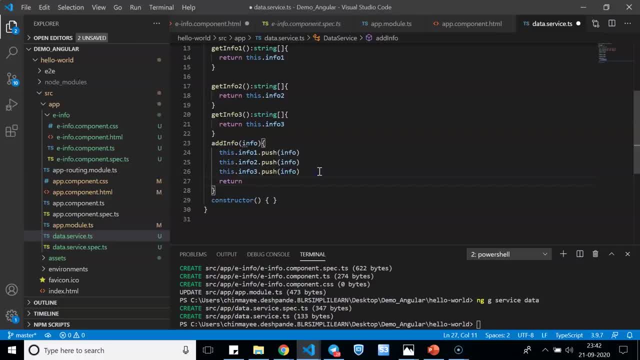 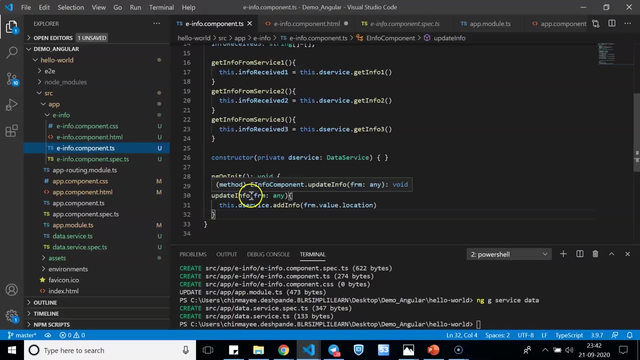 the array and also I have to return it. so I'll say: return this dot info one, all right, and I'll save it. and here we have another method called update info, which basically calls the add info method in our service and passes the value to it and in my HTML file. also note that the button type here is submit and. 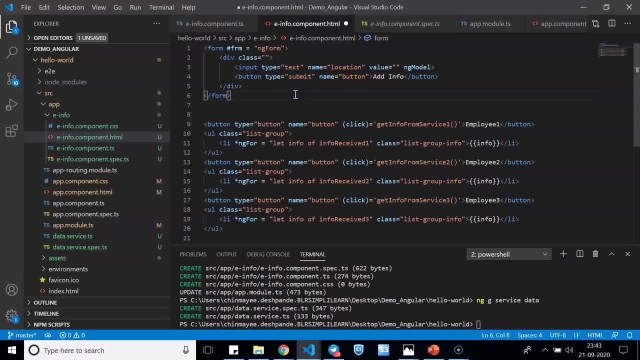 not button. so what happens is that now the value that we've received as an input has to be passed on to the method that is update info. so here I'll say ng submit, and I'm going to call the method update info, and I'm going to pass a forum as the argument. and now let's say this and: 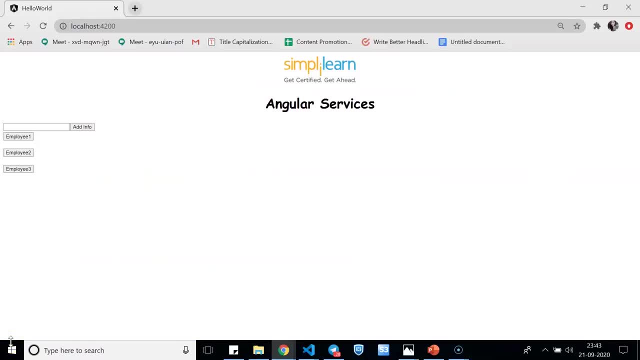 execute. so alright, here you can see that we have an input field and a button seeing add info. so now I can just go ahead and say: type USA, and when I say add info and when I check on my employee, one details: USA has been added to the list. 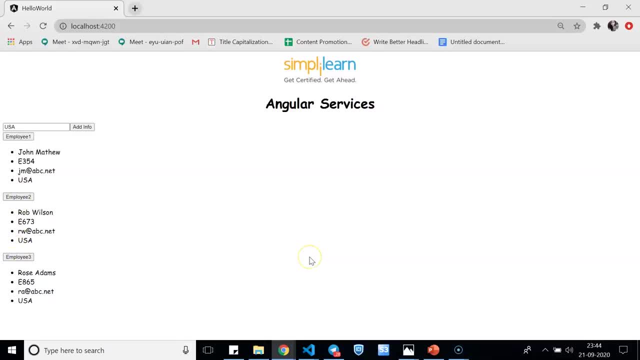 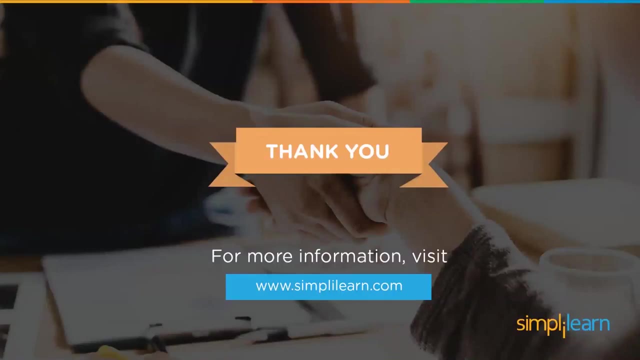 And same goes with employee two and employee three. So I hope this simple demo on Angular services helped you understand the concept better. I highly recommend you play around and explore other possibilities. So with that we conclude the session. I hope it helped you.